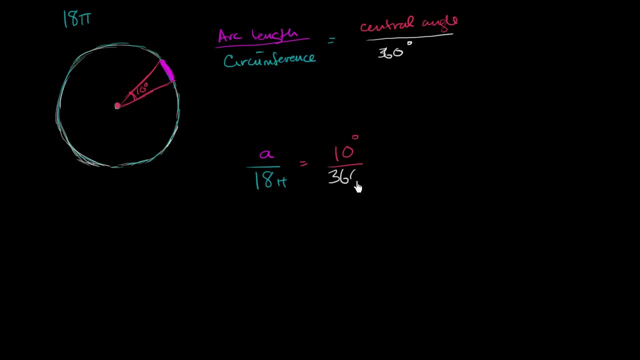 Over 360.. So we could simplify this by multiplying both sides by 18 pi. Multiply both sides by 18 pi And we get that our arc length is equal to well. 10 over 360 is the same thing as 1 over 36.. 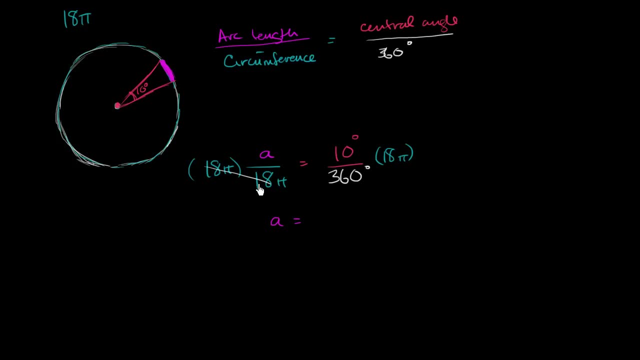 So it's equal to 1 over 36 times 18 pi, which is just so. it's 18 pi over 36.. Which is the same thing as pi over 2.. So this arc right over here is going to be pi over 2,, whatever units we're talking about long. 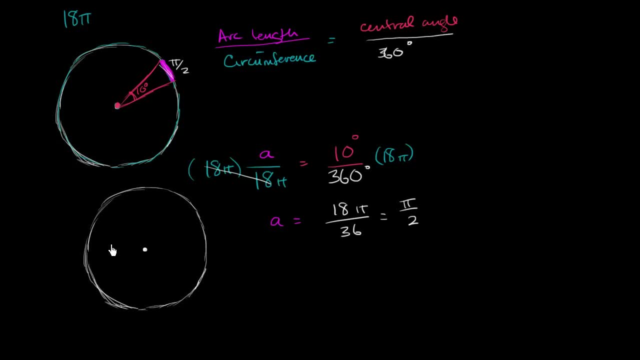 Now let's think about another scenario. Let's imagine another or the same circle. So it's the same circle here. Our circumference is still 18 pi. Circumference is still 18 pi. There are people having a conference behind me. 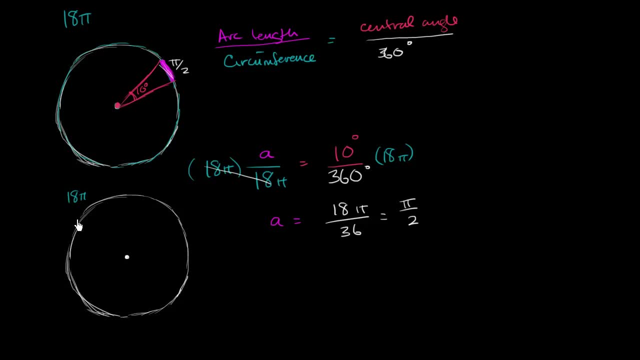 or something. That's why you might hear those mumbling voices. But this circumference is also 18 pi, 18 pi. So this is also 18 pi. But now I'm going to make the central angle, I'm going to make it an obtuse angle. 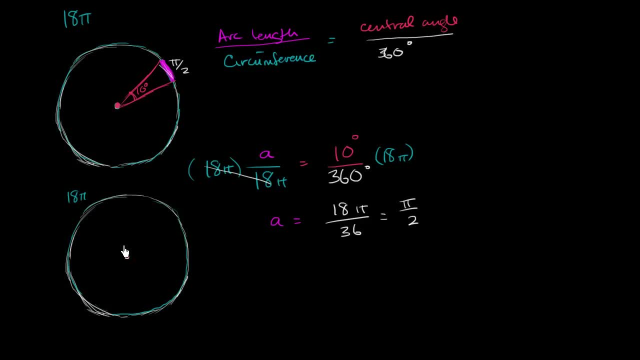 So the central angle now. so let's say we were to start right over here. This is one side of the angle. I'm going to go and make a 350 degree angle, So I'm going to go all the way around like that. 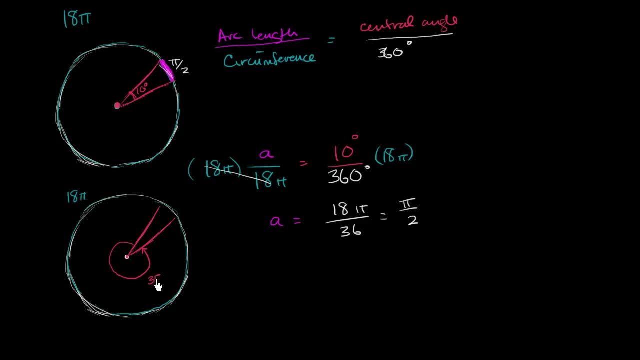 So this right over here is a 350 degree angle, And now I'm curious about this arc that subtends this really huge angle. So now I want to figure out this arc length. So all of this, I want to figure out this arc length. 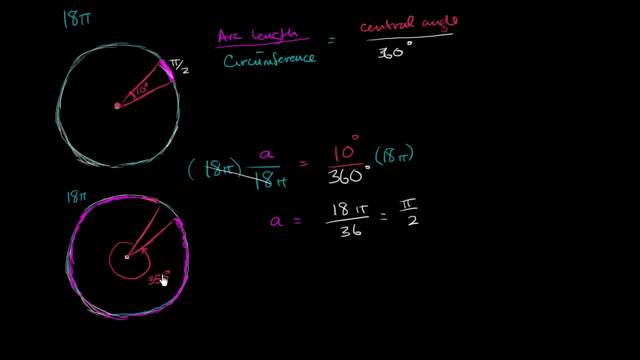 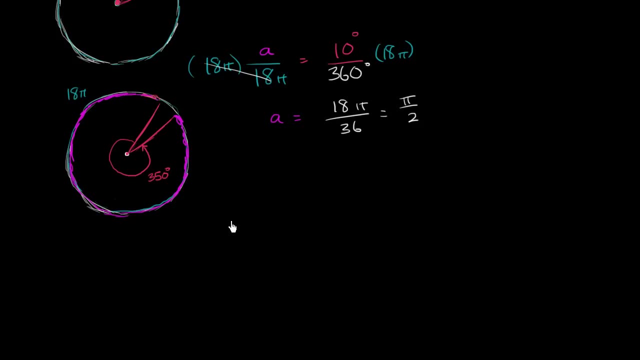 The arc that subtends this really obtuse angle right over here. Well, same exact logic. The ratio between our arc length a and the circumference of the entire circle 18 pi should be the same as the ratio between our central angle, our central angle, that the arc subtends. 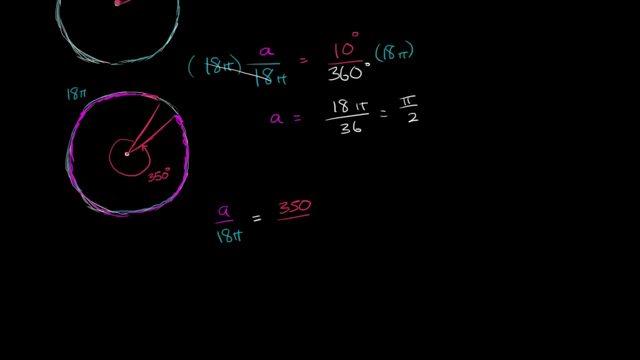 so 350, over the total number of degrees in a circle over 360.. So multiply both sides by 18 pi, we get a is equal to. let's see this is 35 times 18 over 36 pi. So let me. this is so 350 divided by 360.